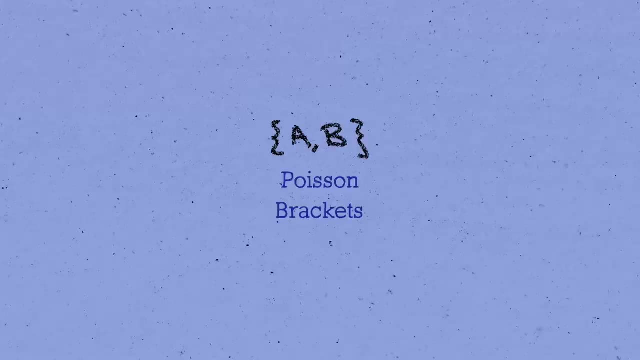 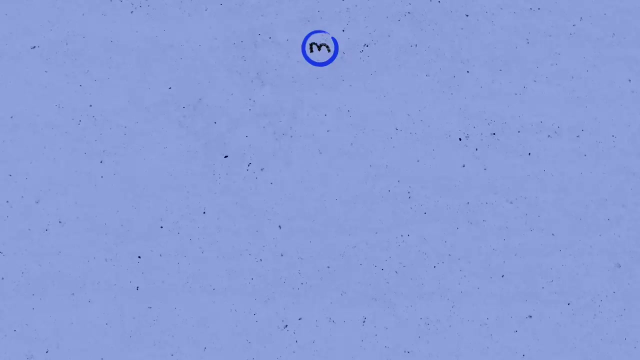 which will hopefully demystify some of these quantum relations or will at least make them look a little more natural when you do start in on your study of quantum mechanics. Let's say we have a particle of mass m with coordinate x. Its equation of motion in other. 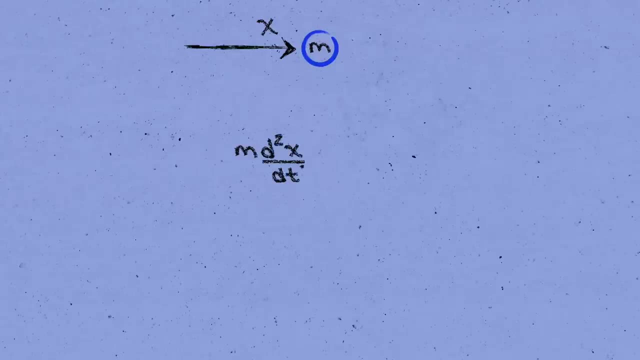 words, the f equals ma. equation is given by m times. the second derivative of x with respect to time equals minus the derivative of u with respect to x, where u here is the potential energy function and the force is given by minus its slope. 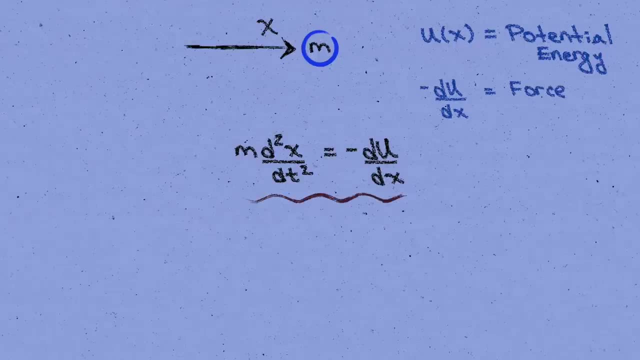 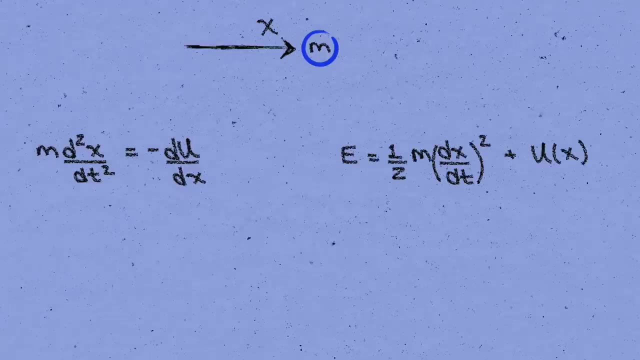 The Poisson bracket is going to enable us to write this equation in a more suggestive way. Let's first of all write down the total energy of the particle, That's one half mv squared where the velocity is dx by dt, plus u, the potential energy. Actually, it's convenient. 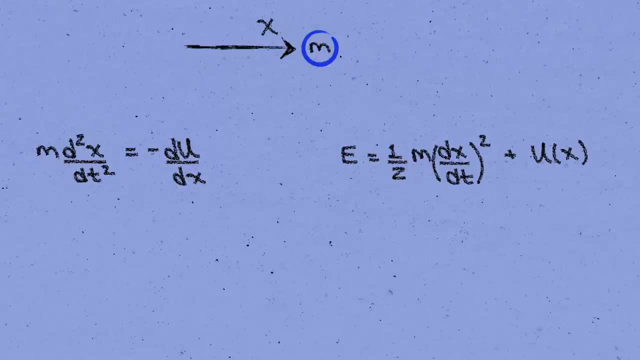 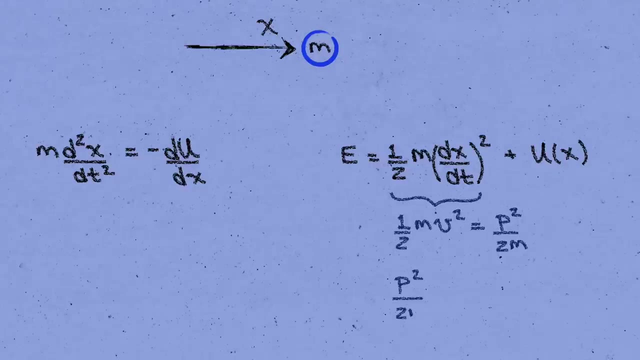 to write this instead: in terms of the momentum, p equals mv, Then the kinetic energy, one half mv squared, can be rewritten as p squared over 2m, And so we get p squared over 2m plus u. This quantity is called the Hamiltonian of the system, and notice that I've written it here. 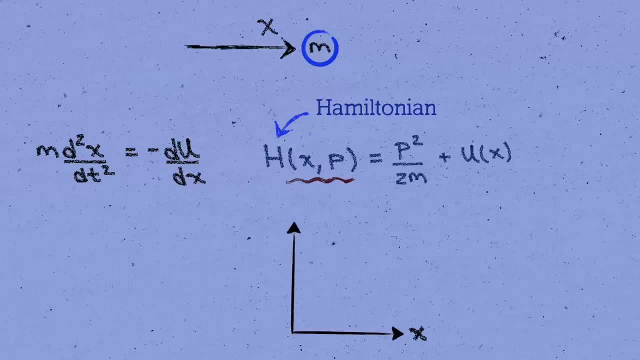 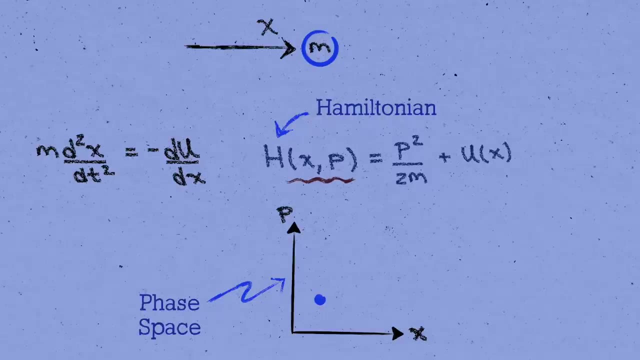 as a function of x and p. The xp plane is called the phase space of our system, and specifying a point in the phase space tells us what the particle is doing at any given instant. After all, giving the position and momentum of the particle at a particular time is equivalent. 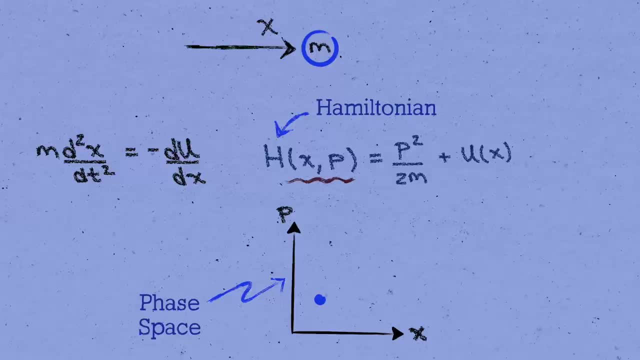 to giving its position and velocity, and those are the initial conditions that we need in order to solve the equations of motion and determine the trajectory of the particle as a function of time. The quantities that we might like to measure about the particle are functions on this space. 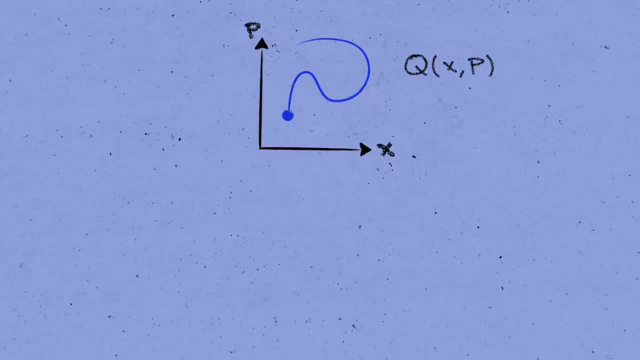 of x and p. Let's denote a generic one by q, For example. we might take q equals x to be the position, or maybe the kinetic energy p squared over 2m, or the total energy q equals h, or anything else. With all that in mind, I'm now going to write down the definition. 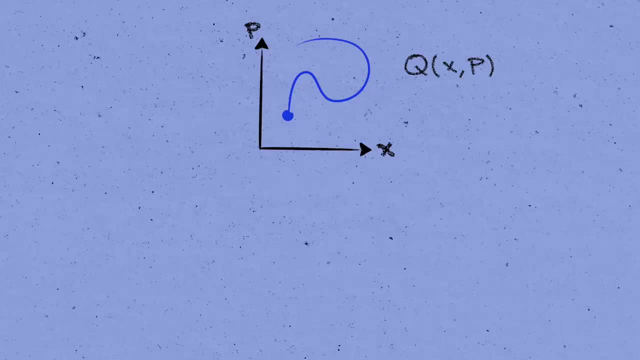 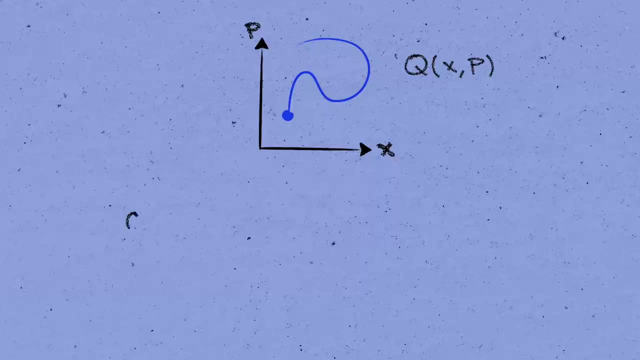 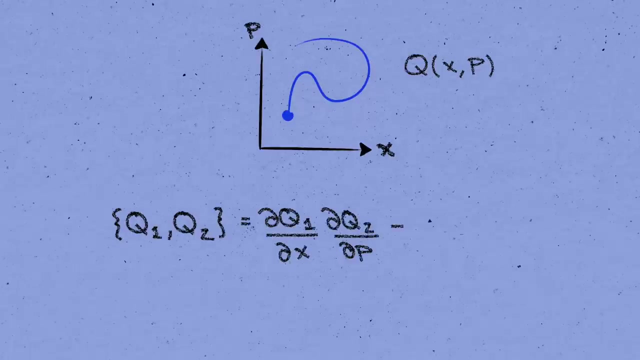 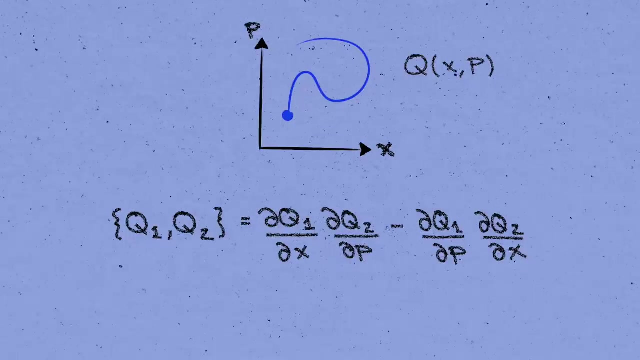 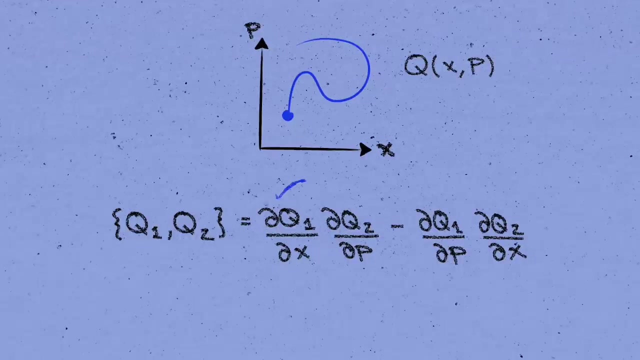 of the Poisson bracket. It might look like a totally random expression at first, but bear with me, we'll quickly see how useful it is. It's a sort of multiplication that we can use to calculate the equation. Q1 and q2 say and returns another. We'll denote it by these curly braces and it's given by the derivative of the first thing, q1, with respect to x times the derivative of the second thing, q2, with respect to p, minus the reverse derivative of q1 with respect to p times the derivative of q2 with respect to x. I'm using partial derivatives here because q1 and q2 depend on two variables: x and p. in general, The partial derivative symbol just. 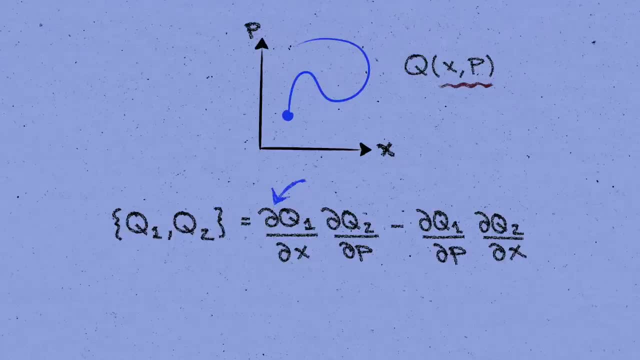 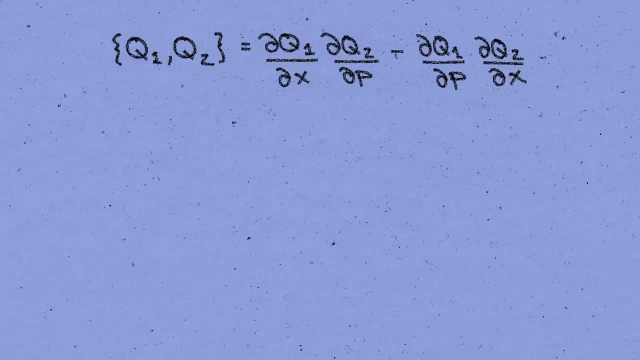 means that we differentiate with respect to each variable independently. Well, that looks a little odd, so let's quickly get at some specific examples to find out why the heck this thing is useful. Say we let q1 equals p be the momentum and q2 equals h be the Hamiltonian. Then their 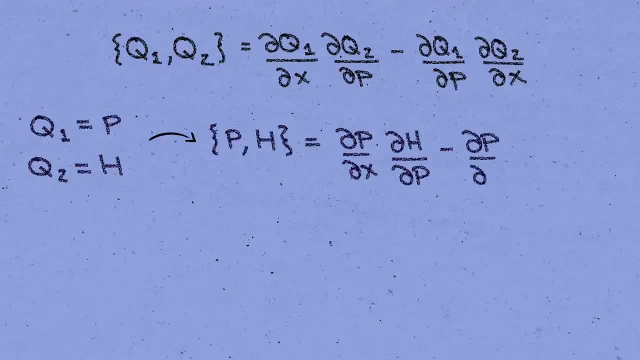 Poisson bracket is given by dp by dx times dh by dp, minus dp by dp times dh by dx. Right off the bat, the first term is zero. p and x are independent variables, and they're independent variables here, and so the derivative of p with respect to x vanishes. As for the 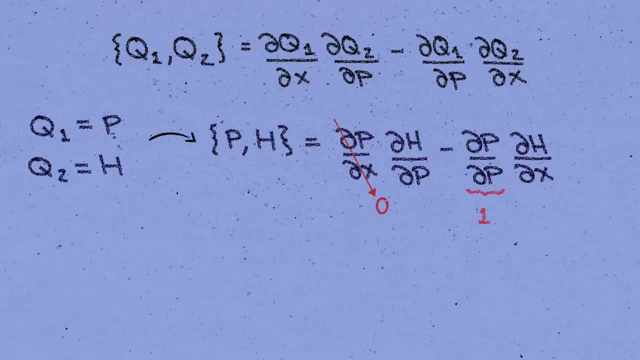 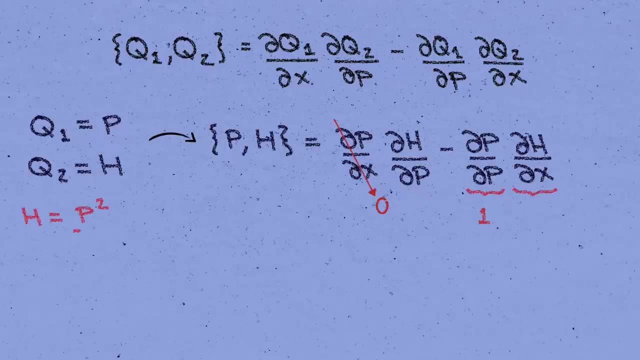 second term, the derivative of p with respect to itself is of course 1, and as for the derivative of h with respect to x, remember that we defined the Hamiltonian as: h equals p squared over 2m plus the potential u, And so the x derivative only gets a contribution from the potential. 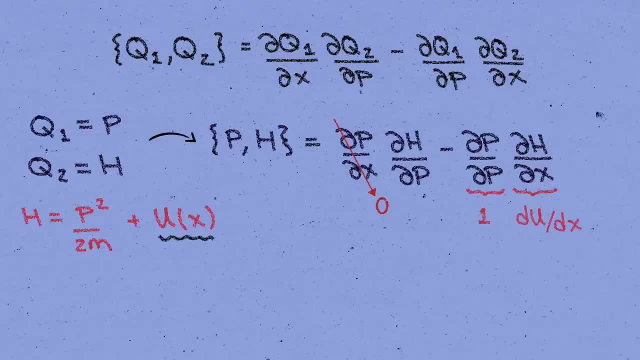 term du by dx. Therefore the Poisson bracket of p with h is equal to minus the slope of the potential. But we can write this more suggestively by remembering that that's just equal to the force on the particle, And by Newton's second law, the force equals the rate of change. 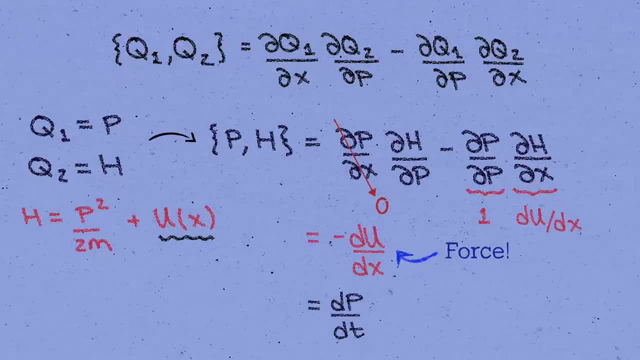 of the momentum dp by dt. Therefore, we learn that we can rewrite Newton's second law as the statement that the rate of change of the momentum p is equal to its Poisson bracket with the Hamiltonian h. That's a cute way of rewriting: f equals ma. So maybe we're onto something here, Or maybe 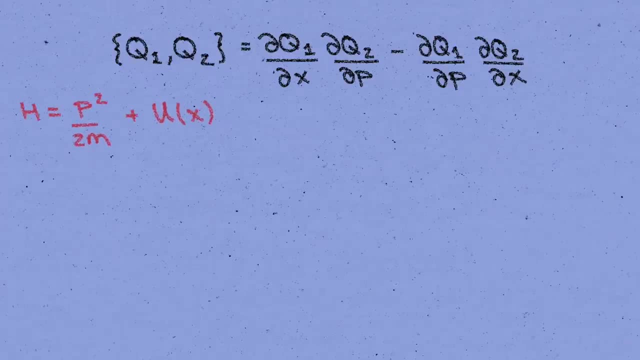 it's just a fluke. Let's check another example: What's the Poisson bracket? So what we get is the Poisson bracket of x. with h. We get dx by dx times dh by dp, minus dx by dp, dh by dx. This time it's the second term that vanishes, because the 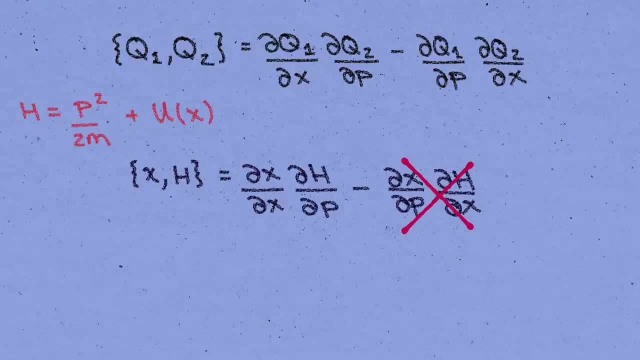 derivative of x with respect to p is zero, Then in the first term the derivative of x with respect to itself is 1, and the derivative of h with respect to p comes from the kinetic energy term in the Hamiltonian, p squared over 2m, So we get p divided by m for that. 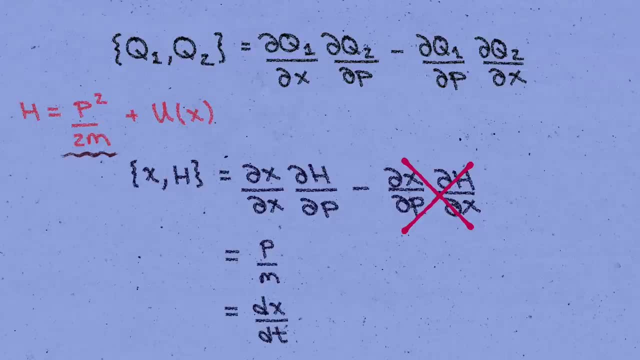 derivative That's just the velocity of the particle, dx by dt. So we've obtained a similar relation that the rate of change of x is equal to its Poisson bracket with the Hamiltonian. By the way, if you find yourself a little tangled up by all these derivatives, I strongly 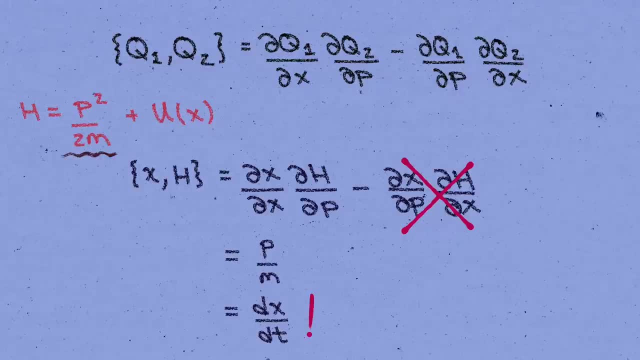 encourage you to work through all these equations for yourself with pencil and paper To help. you can get the notes that I wrote up for this video for free at the link in the description. But okay, this isn't looking like a coincidence anymore. 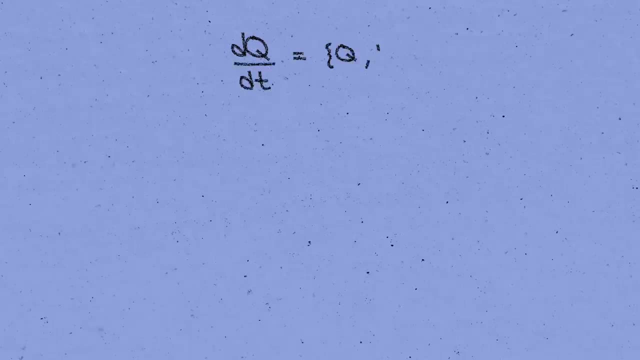 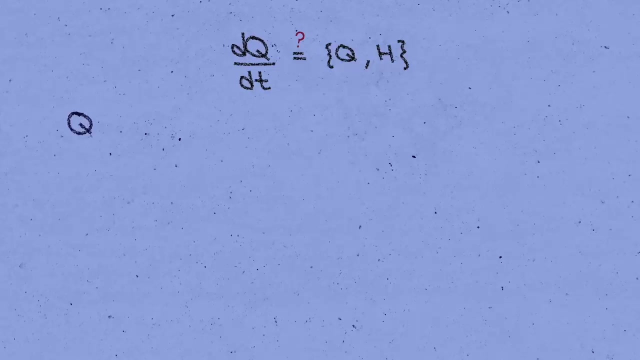 Is there a general relation here that the rate of change of any function q on face space is given by its Poisson bracket with the Hamiltonian? Well, let's check. As time goes by, q and p will in general be changing because x and p are changing. 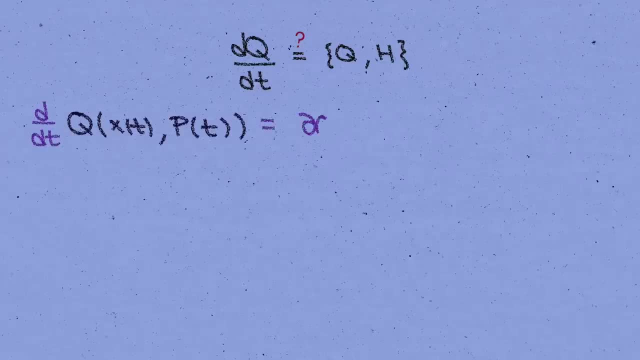 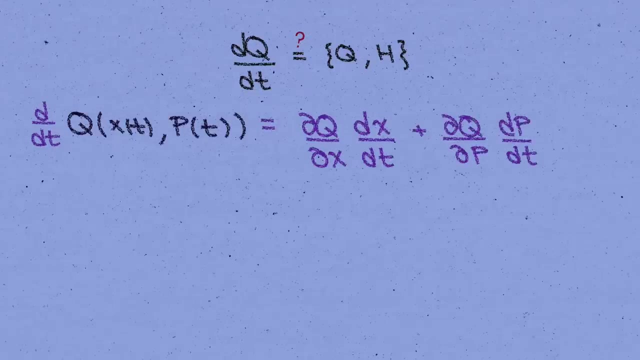 And we can get the rate of change of q by applying the chain rule. First we take the derivative of q with respect to x and then multiply by the rate of change of x, And likewise we take the derivative of q with respect to p and multiply by the rate. 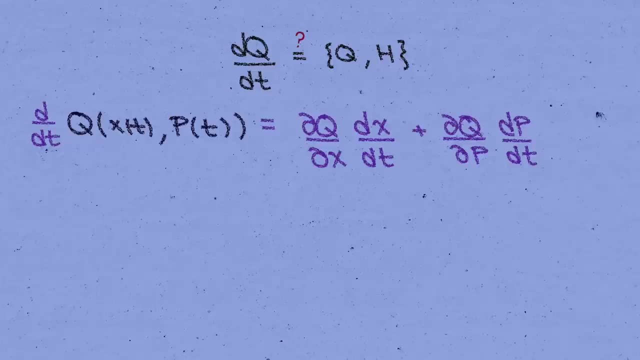 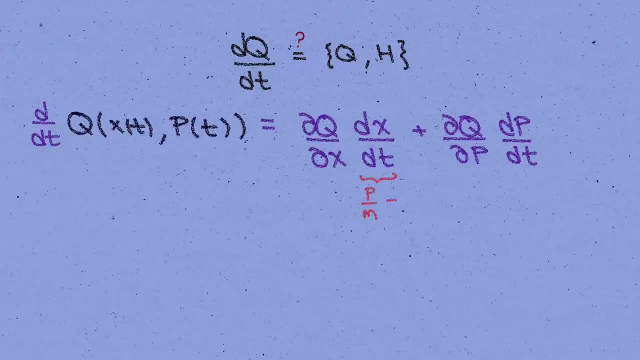 of change of p. Then we add them up to get the rate of change of q with respect to time. Well, we've seen all this And we'd like to write them as derivatives of h. dx by dt is the same as p over m, and we just saw that that's the same as dh by dp. 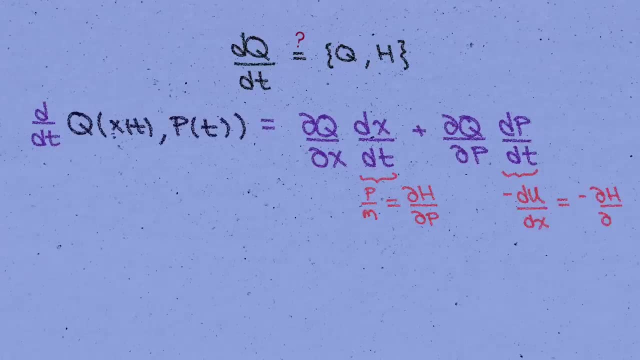 Meanwhile, dp by dt equals minus the slope of the potential, which is the same as minus the derivative of h with respect to x. So we learn that the rate of change of q is dq by dx times dh by dp, minus dq by dp dh. 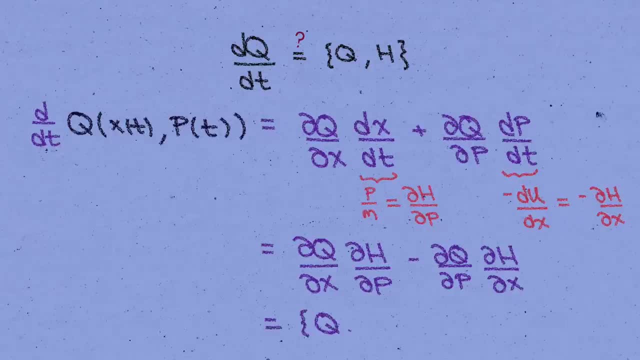 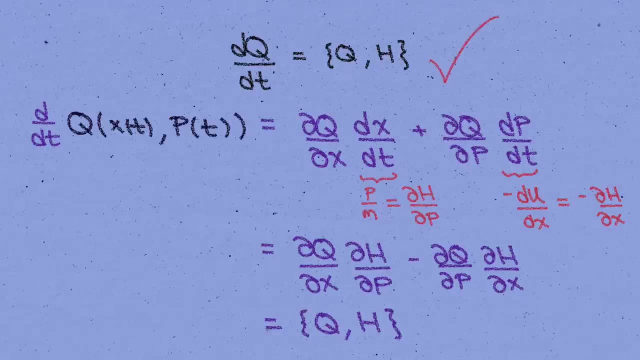 by dx, But now the right-hand side. here is precisely the Poisson bracket of q and h. So we've discovered that this is indeed a very general relationship. The rate of change of a function, q, with respect to time is given by its Poisson bracket, with. 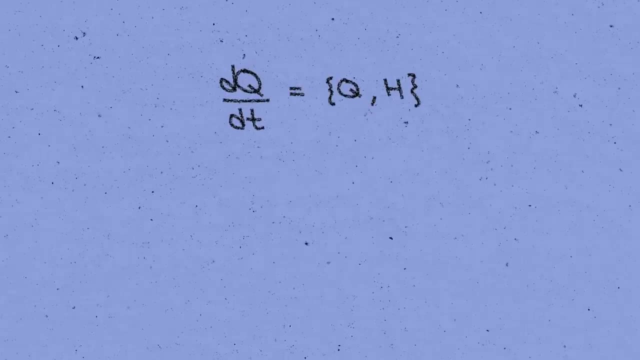 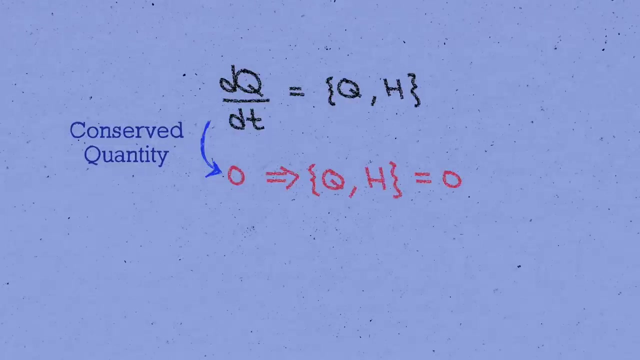 the Hamiltonian, And this is a beautiful result. Notice, for example, as a special case, that for a quantity that's conserved, dq by dt is equal to zero, and therefore the Poisson bracket of q with h must vanish. 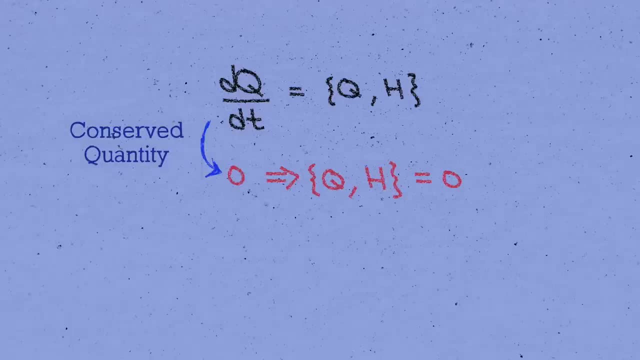 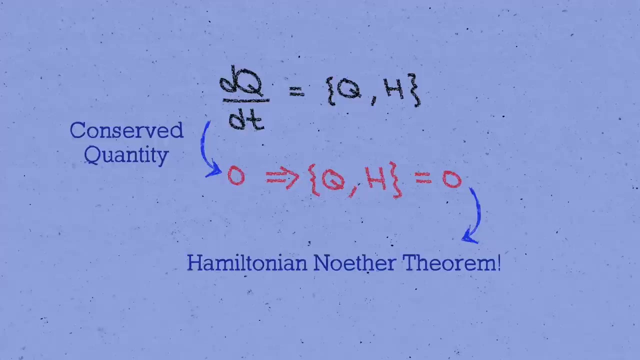 Although that make sense, which is the 뜻 of this equation, also means that the timber can mutate another layer by a simple force of force sine equal to the point h over y times ratio. If you'd like to see that explanation in a future video, comment below. 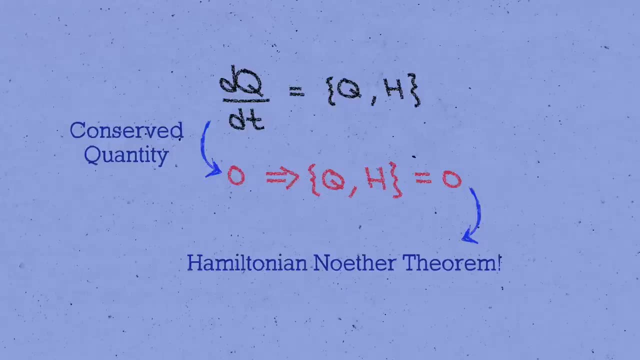 It's a bit more advanced than the Lagrangian version of Noether's Theorem, which I covered in a recent video, but it's even more beautiful. 魔法歌, Thinking back to where we started a few minutes ago, the thing that's hopefully jumping. 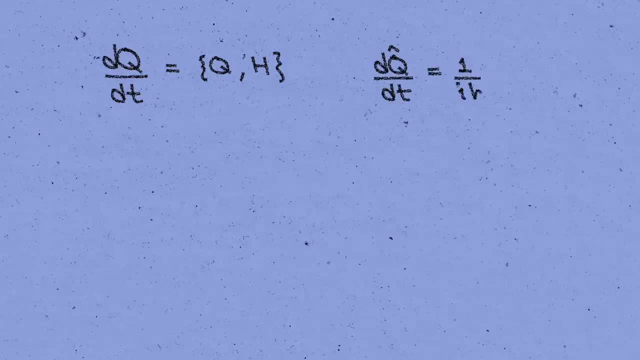 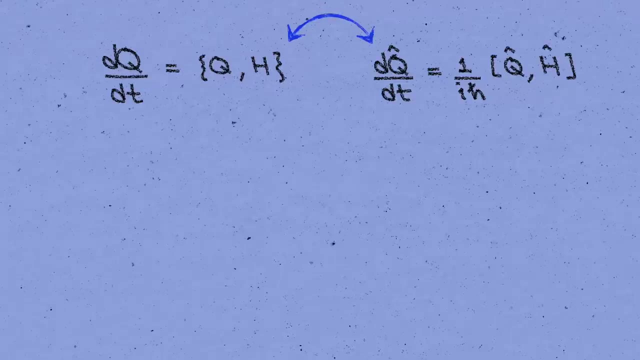 out at you is that this equation is remarkably similar to the Heisenberg equation of motion for a quantum operator. We're not going to delve too deep into the general rules of quantum mechanics in this video, but the gist is that functions on the classical phase space like 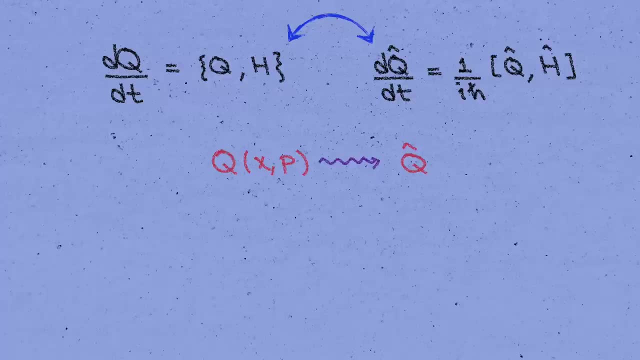 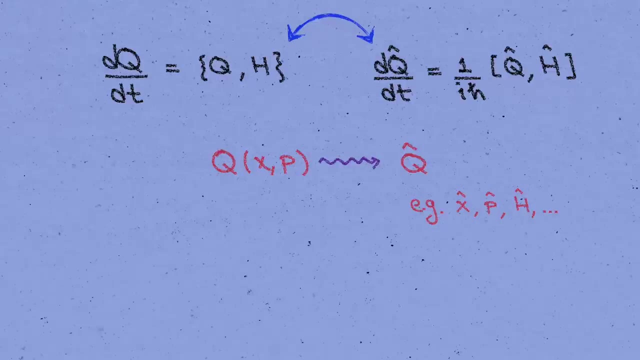 q turn into operators acting on the quantum wavefunction. For example, we've got the position operator x-hat, the momentum operator p-hat and the Hamiltonian operator h-hat, and so on. That's what the hats indicate here. q-hat is the quantum operator corresponding. 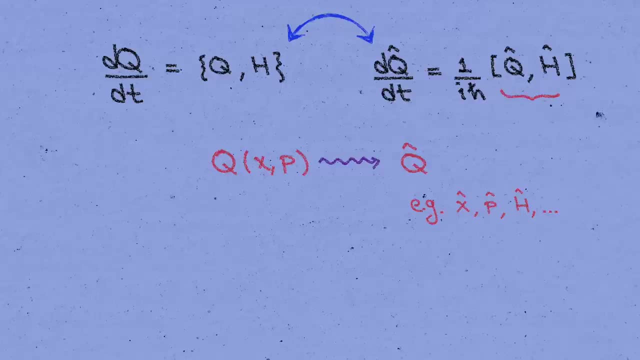 to the classical function q. The square brackets, like I mentioned at the top, denote the commutator of two operators, q-h minus h-q, And the order matters here. These operators are like a generalization of matrices, And when you multiply matrices together you'll get different answers in. 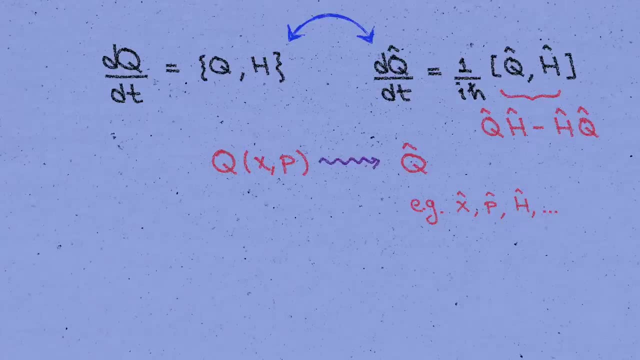 general if you combine them in the opposite order. If you've never seen Heisenberg's equation of motion before now, you will when you start studying quantum mechanics. For the moment, I just want you to notice the remarkable parallel to our Poisson bracket.